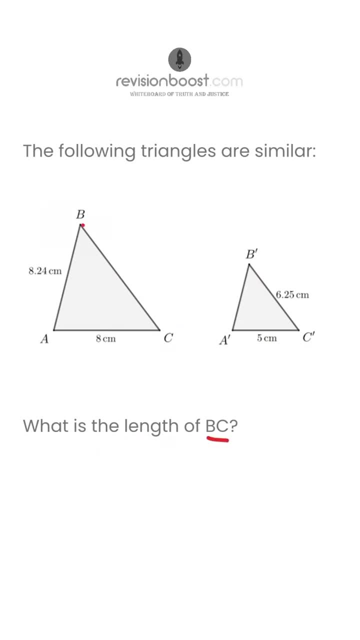 Then from this we're asked to find the length BC which, as you can see from the diagrams, is this length? here, On similar shape questions like this, the key is to find the scale factor between the triangles. You can do this by taking the length of two corresponding sides. that you know, and 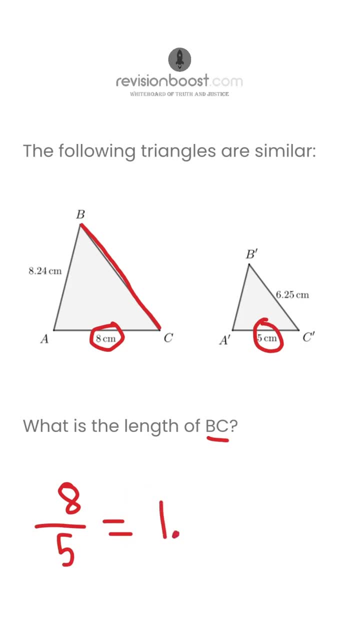 dividing them. So in this case I'll do 8 divided by 5, which is 1.6. so this is the scale factor. As a result, I can find the length of this unknown side by taking the corresponding side on the small triangle and multiplying by 1.6.. 6.25 times by 1.6 is 10, so BC has a length of 10 centimetres. Thank you for watching. 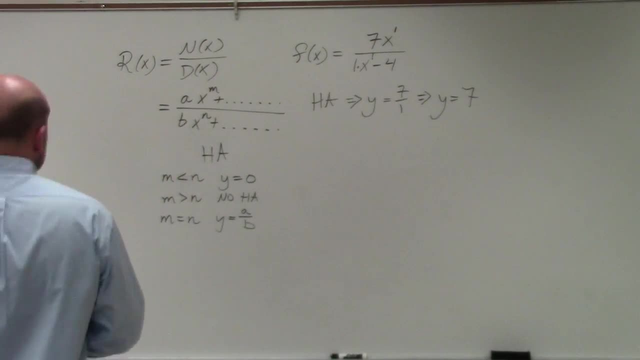 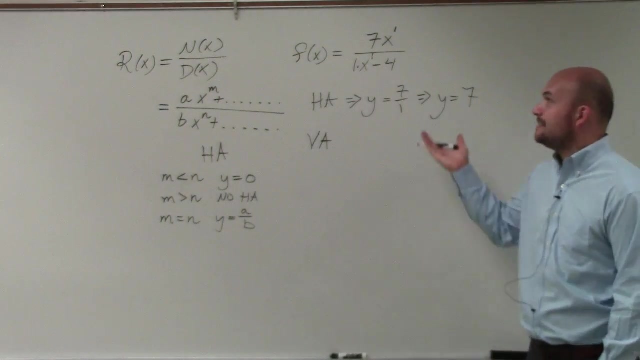 I'll just might as well do both As finding the vertical asymptote. to find the vertical asymptote, basically, all we're simply going to do is take the denominator and set it equal to 0. And this is something that's going to be really, really important. next chapter: 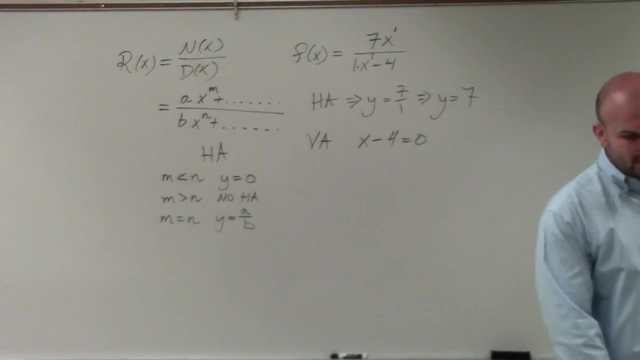 once we start getting into our limits, Because when we're looking at this, we know that we can't divide by 0, correct, We cannot divide by 0. So our vertical asymptotes are going to occur when we have values that are not. 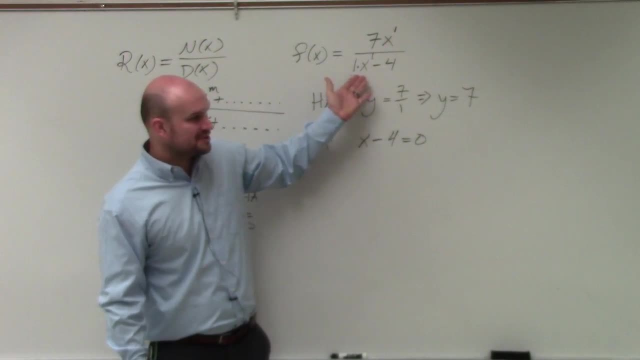 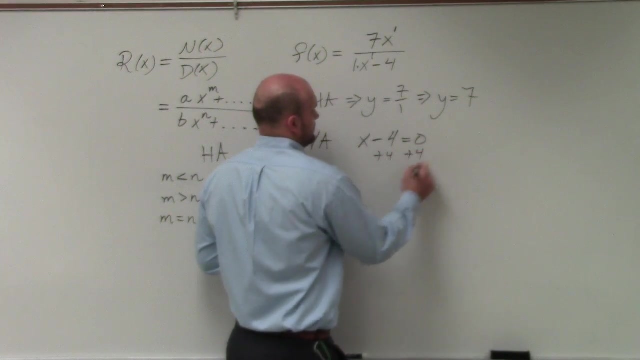 inside the domain, which would be values that would make our denominator equal to 0.. So to find the vertical asymptote, all you simply need to do is set your denominator equal to 0, and then solve: x is equal to 4.. 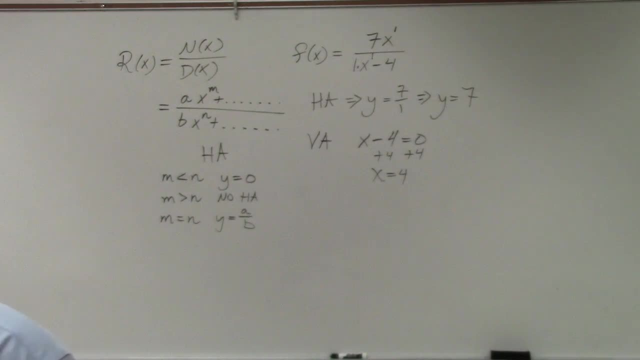 And that's your vertical asymptote. I know it didn't.